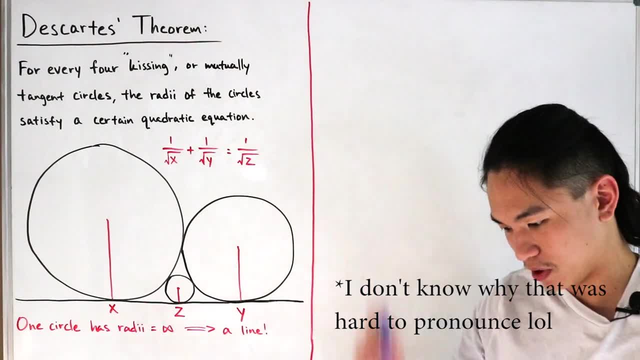 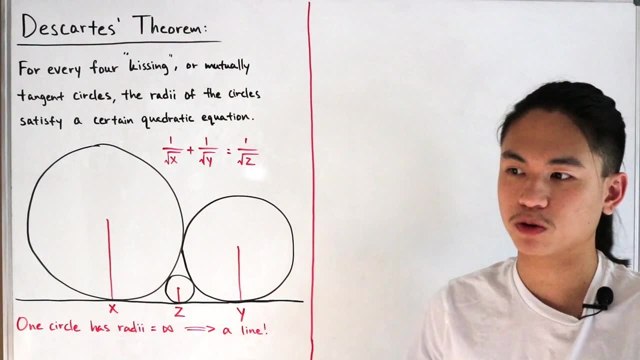 theorem. So that would be important, And it's just a whole lot of manipulation from there and it's actually pretty straightforward once you once it comes down to the final conclusion. So anyway, let's just start. So let's actually do a little bit of construction over here. 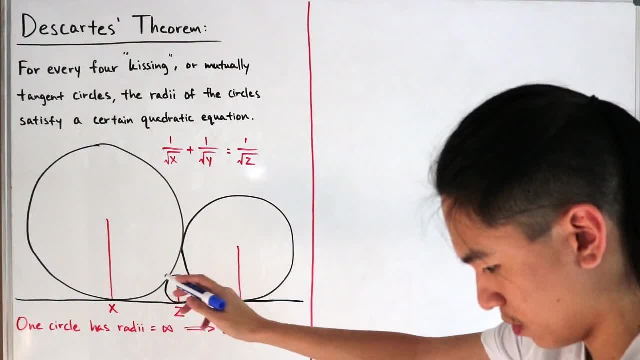 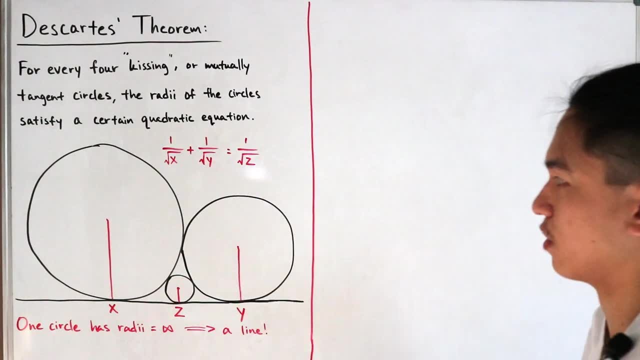 So what I'm gonna do is I'm actually going to draw some. I'll call I'll the way. I'll list. it is like dotted lines, but that's basically just the gist of how the construction works. So I'm just gonna add two line segments, starting with our radius z, but connect the lines to. 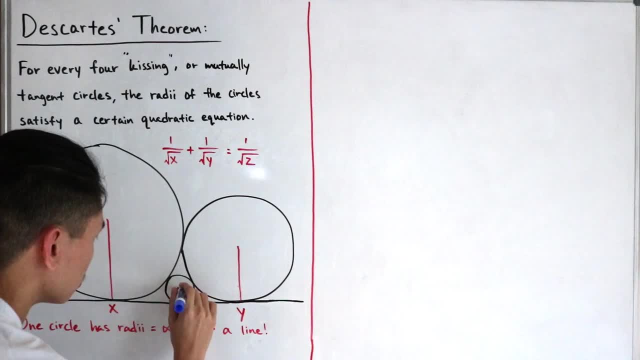 so that's tangent to this line of the radius. So let's see, so that's one. I know it's obviously it's not meant to be perfect, so I apologize for that, but you understand where I'm going with the picture over here, Okay. 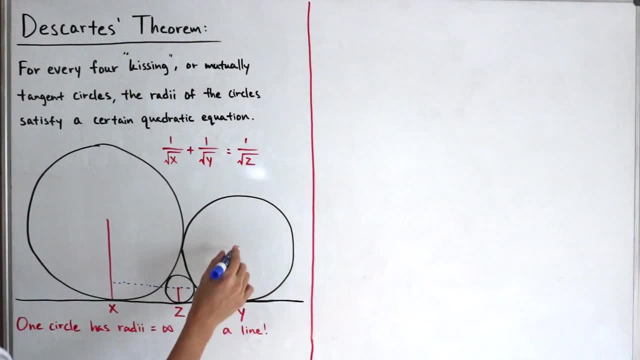 so that's one line segment and then we're gonna connect this, the rate, the center of our radius that has y, and then draw a line segment connecting to all the way to the end of where the line segment of x of the radius is. 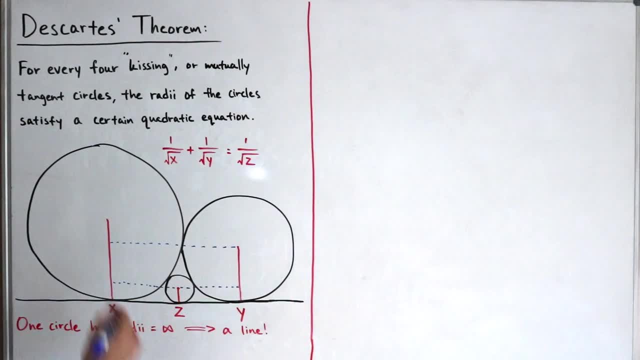 All right, cool, And how about this? I'll actually label these vertices, that's in the connection Of these line segments and the radius, of course. So here I'll just call this a, call this b, we'll call this over here c, and then over here we'll call this d, like so Okay. 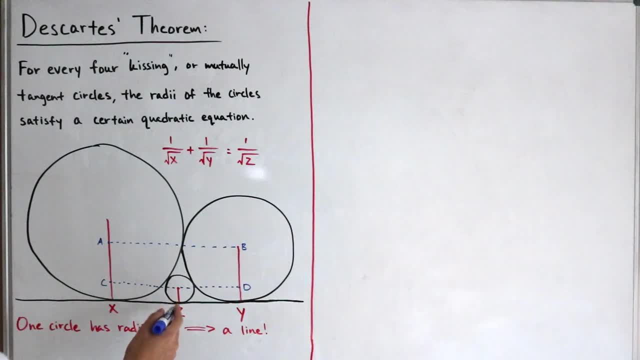 So let's actually continue a little further and actually draw more line segments so that way we actually form a little triangle. So let's see, I'll connect the center of this circle all the way to the connection Of this circle over here. all right, that's one, and then we're gonna connect this over. 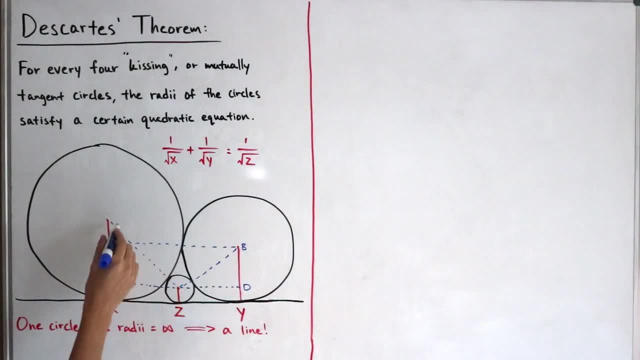 here, right, And then one more, one more circle or one more line segment connecting from this rate to the center of the circle x, x, with x radius, and then the center of the circle with radius y. Okay, so we have that. So I'm actually going to fill in the fill in our 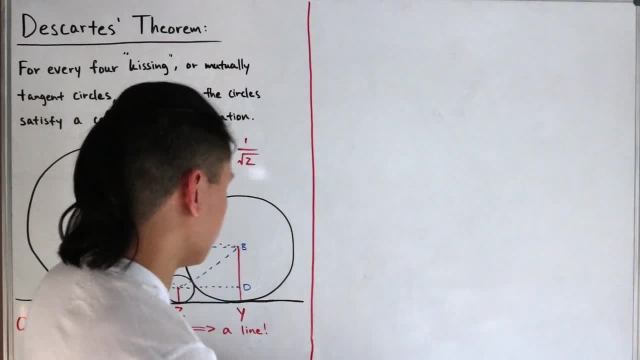 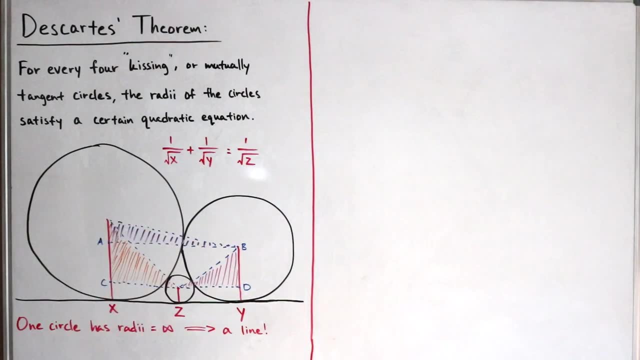 triangles with the different color. So give me one second to do this. So here's our little little construction of our circle. So now let's actually denote some of the the lengths of these of the line segments over here. All right, so first off, we see that the line 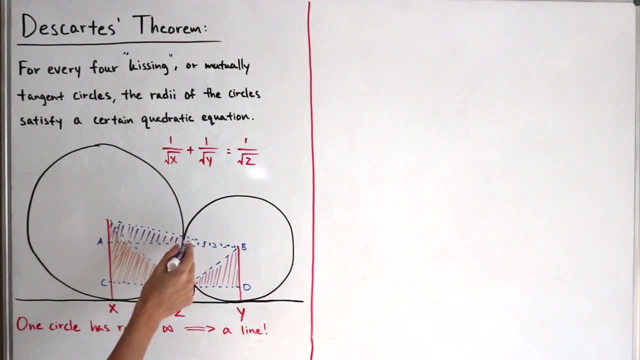 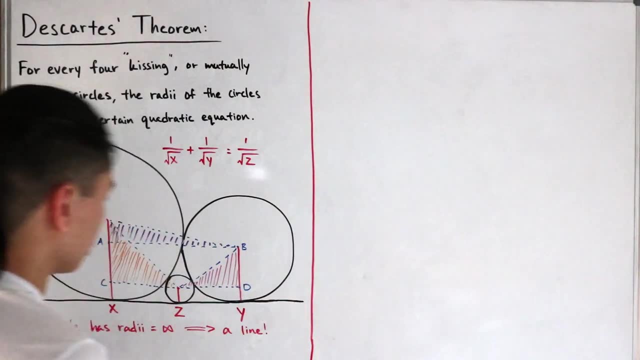 segment connected from here to here. Notice that this is actually just a sum of the radius from x and then y. So I got a better idea. So here I'm actually going to draw up some triangles here. So here we have our first triangle. This is just a basic triangle, but 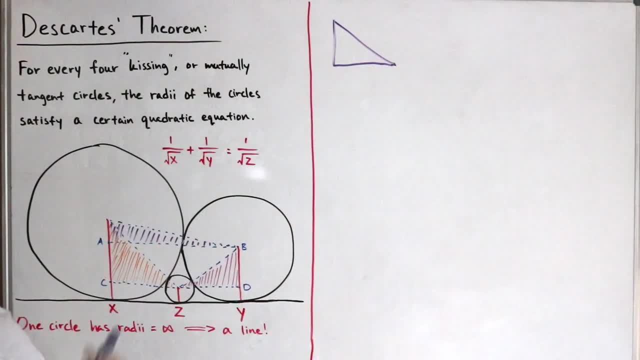 the lengths, the length of these, the sizes would matter. The first part is the purple triangle shaded. So I drew, you know, a purple, a triangle in purple color. So we know that. we noticed that the hypotenuse over here would have to. 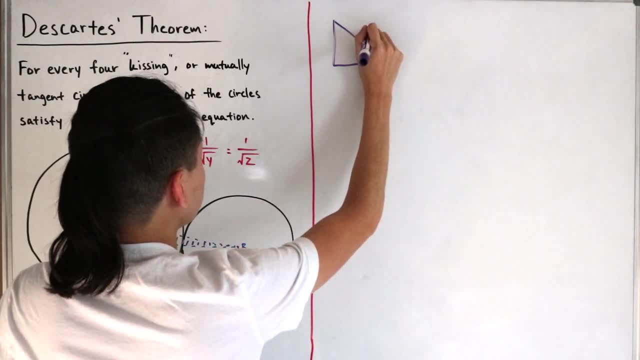 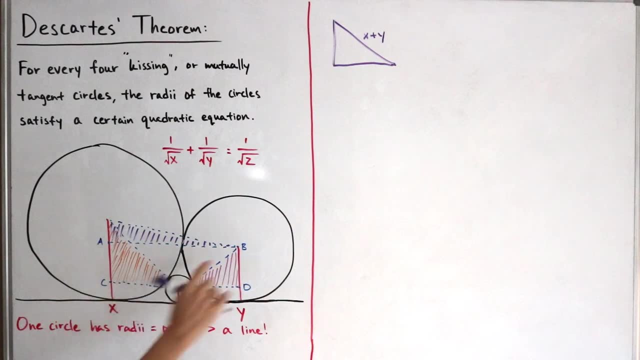 be the sum of the um, the segments of the of the radius, So this will be x plus y, Then over here from the sum, so it's connected to x, and then subtract from the length from here to here, So it's x minus y Um. so that leaves us with an unknown base. So now let's. 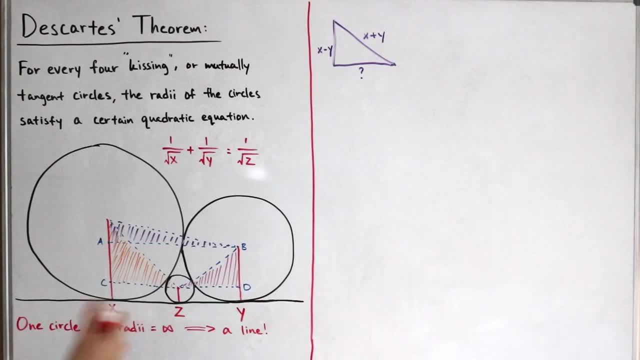 calculate the second triangle. Well, not calculate the triangle, second triangle yet, But like, let's actually denote its lengths. So here I have, next up orange triangle, And we know that the hypotenuse from here is that this is connected from the radius of x or 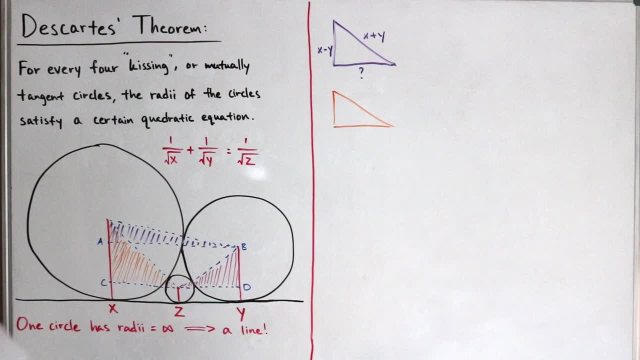 from here and then add that with the length of y of z, So that's the orange, the orange triangle. hypotenuse is actually hypotenuse. length is x plus z. And then, from over here, going back to that same triangle, we noticed that the length, or the height rather, is connected. 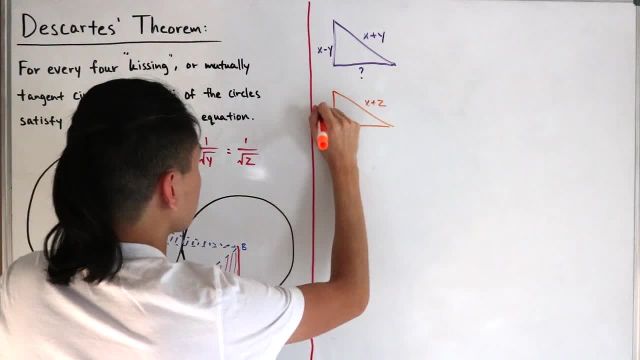 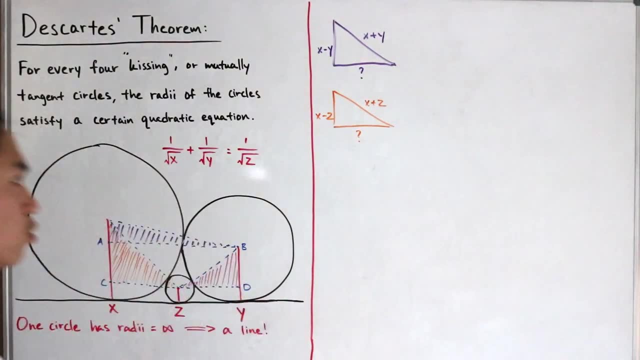 from x, then subtract with the length of z, So this will be x minus z, with an unknown base. And then the last part is the one pink, So triangle in pink. I know it's backwards with reflection, but again what matters is: 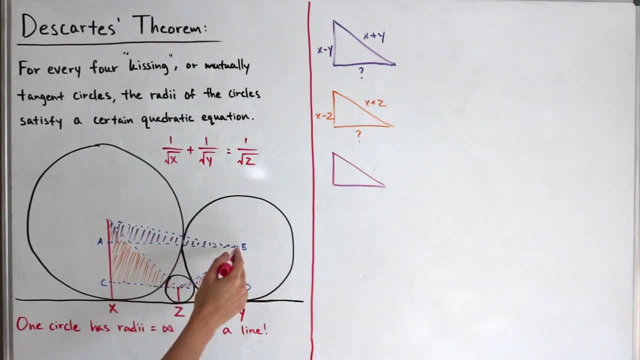 the length of our sides. So we see that the length of the hypotenuse is um, connected with um length of y, the radius from this circle, and add that with the link of the radius from z, So it's hypotenuse would be uh, y plus z, And then we see from here. 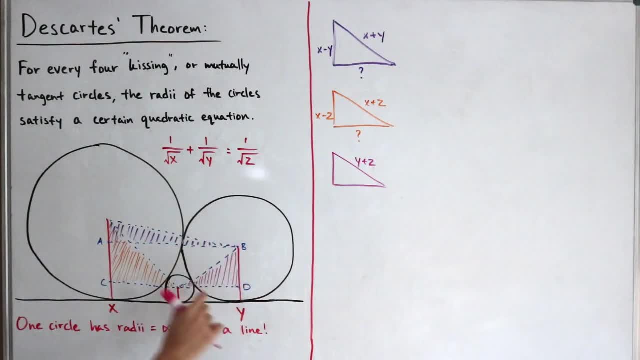 with um, the height of the pink triangle is from y, then subtract with the length of z, So the height would be y minus z with an unknown base. Okay, So we have those. So now let's actually um find these unknown bases, which, of course, this is actually we, uh. 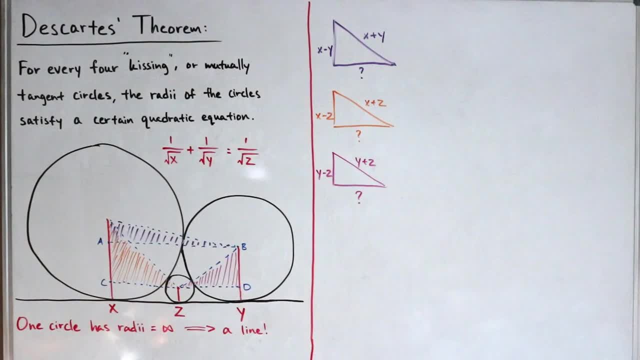 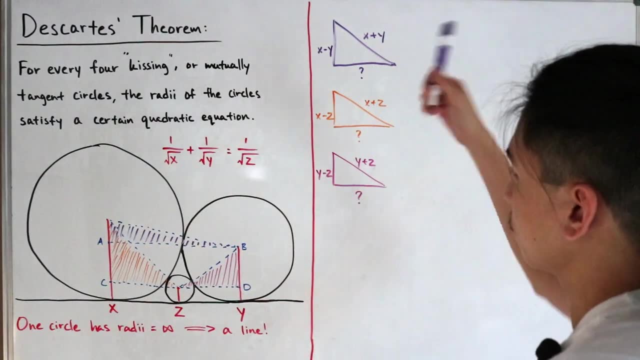 as mentioned, you're going to have to use the Pythagorean theorem. We'll start off one by one and solve these unknown bases. So we know, obviously we all know, that the Pythagorean theorem states that for um, um, when you're solving for the hypotenuse, it's a squared. 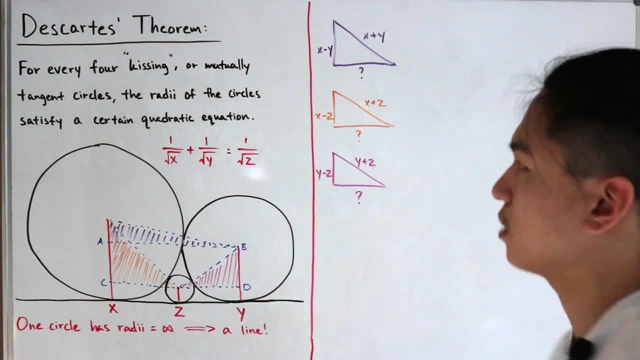 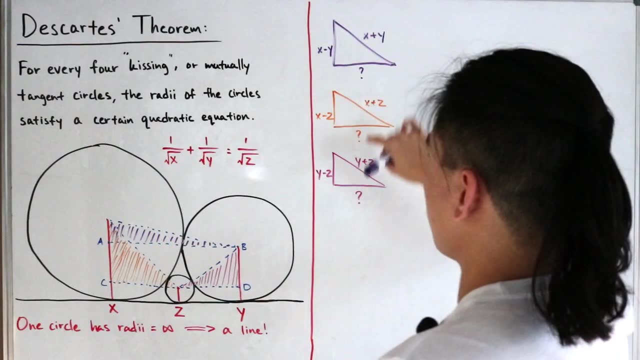 square, which is your base length. Then C square is: C is your hypotenuse length, Since we already know both one of the sides or it's one of the base and hypotenuse. So we have to solve for one of the bases. Again, I'll just call this a for the corresponding three. 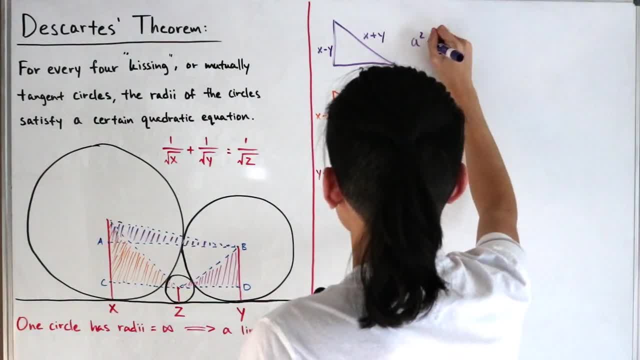 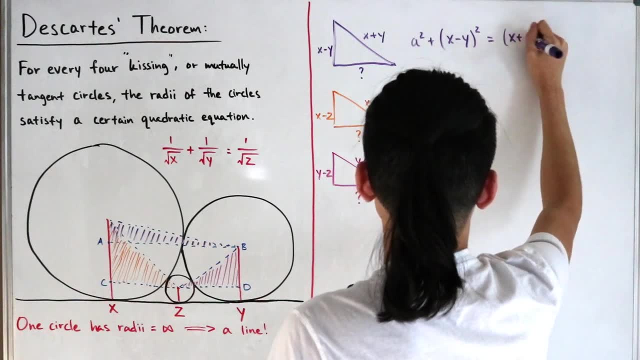 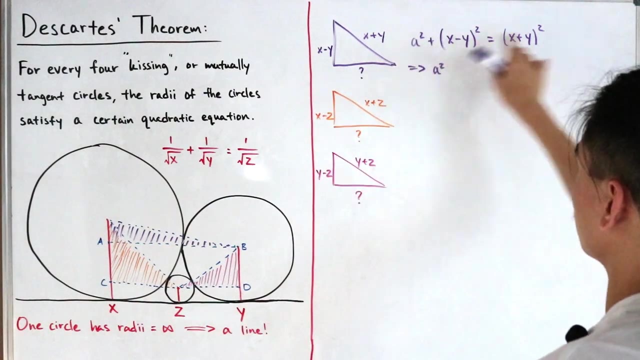 triangles we have to solve. So I would mean a square, then add this with um x minus y square, Then they set that equal to um x plus y square. Okay, So we solve this. This is a square- and I'm actually going to expand this out- but also subtracted. 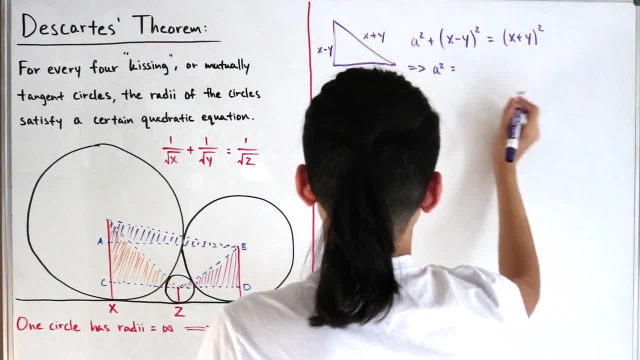 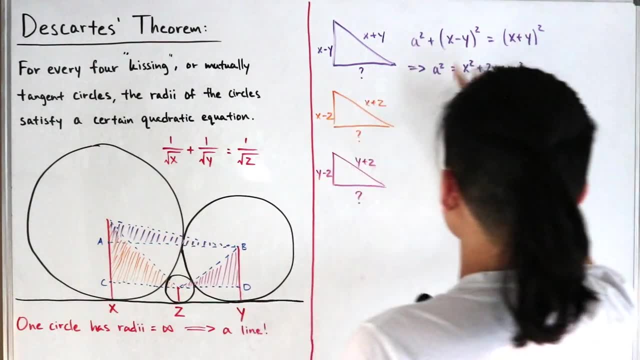 To the other side, since we're actually selling this for a. so let's see if I expand this out. So we have x square plus, uh, two x y, then plus y square, Then this will be: um, this is positive, I subtract, So this will be a minus x square, then a minus, minus. So 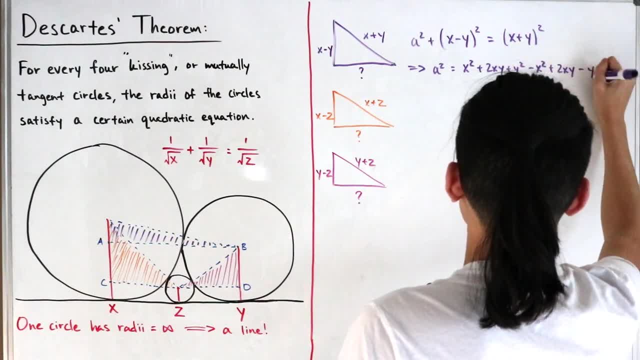 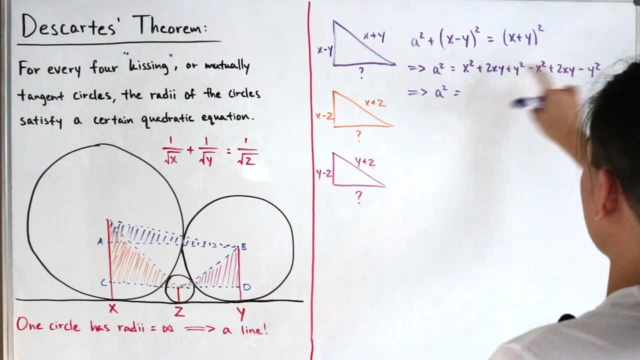 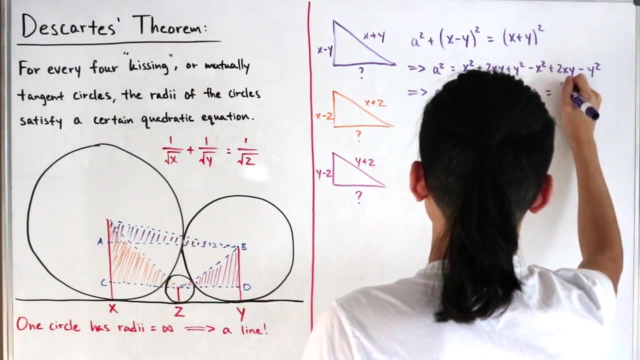 this is positive. two x, y, and then subtract y square, Then we see that um a, a square is equal to, so x squares and x squares. cancel y square, y square, cancel, So it's just four y. Therefore the length of the base is just um. a is equal to, uh, two times the square. 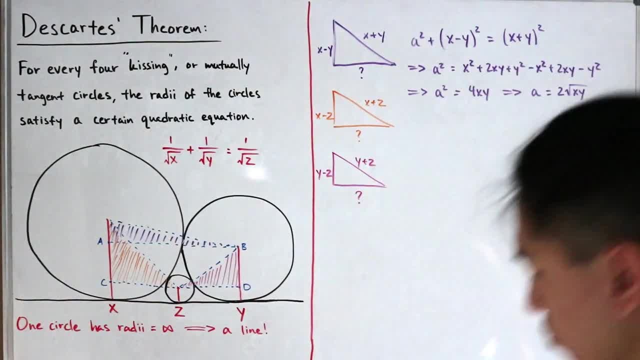 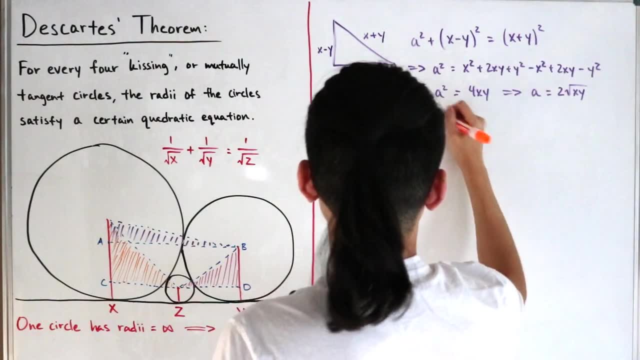 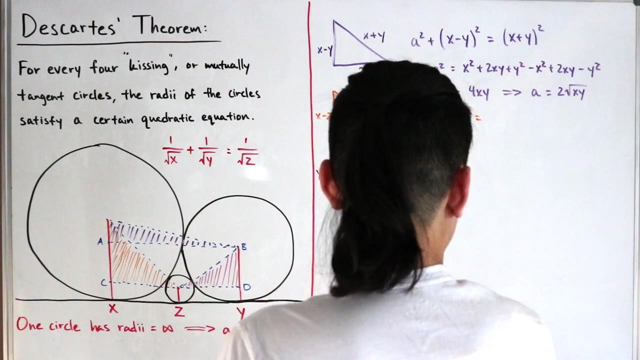 root of x, y. All right, So that's one triangle down. Let's move on to the orange one. It's the same process again. Do the same thing. I said um a square then equals um. x minus z square equals. actually that's supposed to be a plus right here. So plus then um. 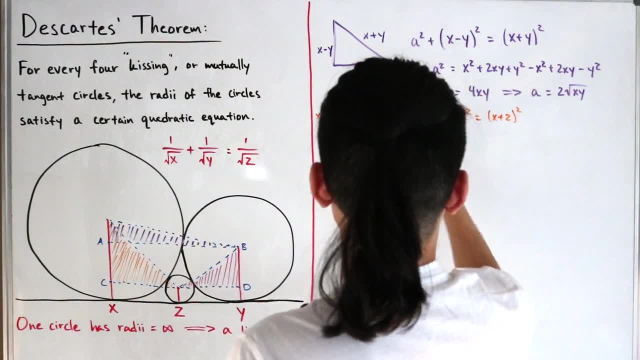 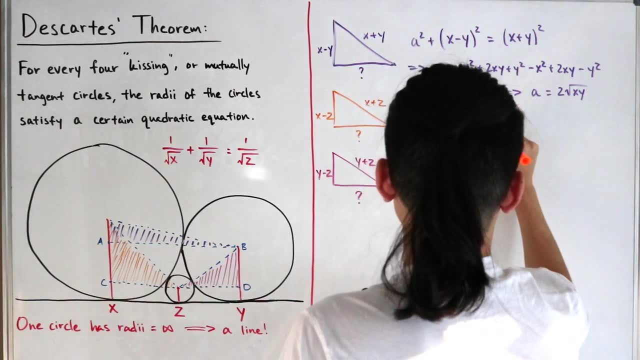 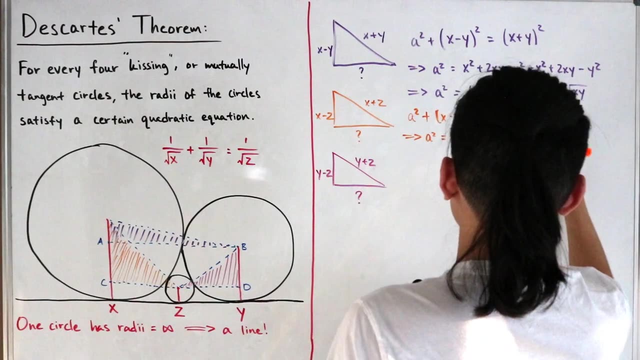 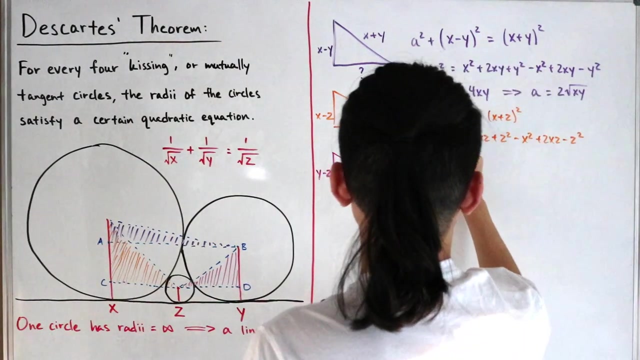 x plus z square. So let's solve this out. Then a square is equal to x square plus two x z plus z square. Then subtract, So x square, that's just subtracting this quantity expanded quality to the other side. Then this is plus two x z. Then, um, subtract the z square, A is equal to well. 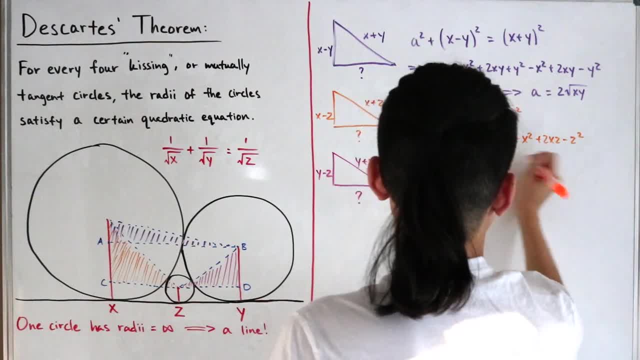 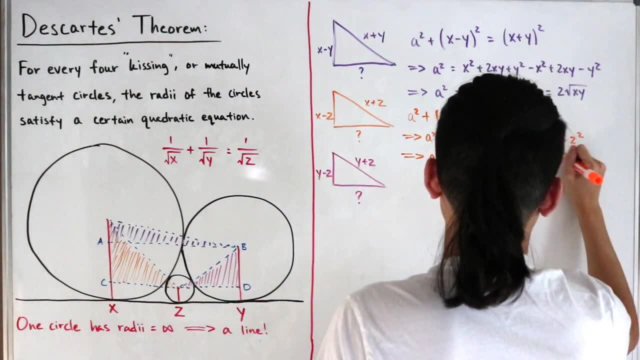 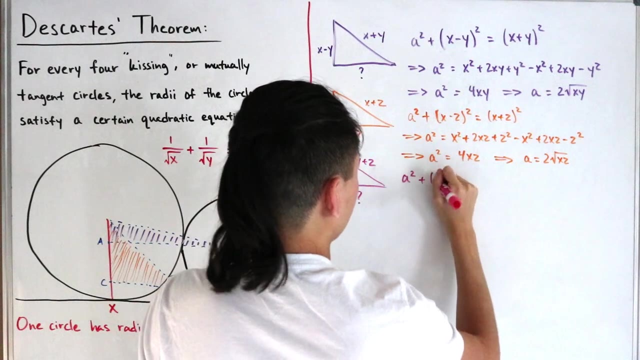 a square is equal to four x, z, And we see that um, this- this base over here, is a- is equal to, uh, two times the square root of um, x times z, And then one more triangle to go And it's um. we have a square then plus y, minus z square. Then we set that equal. 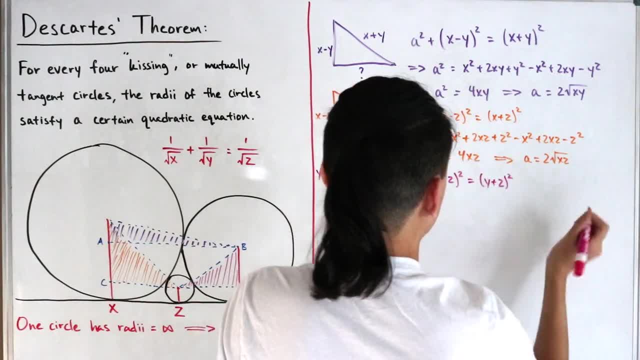 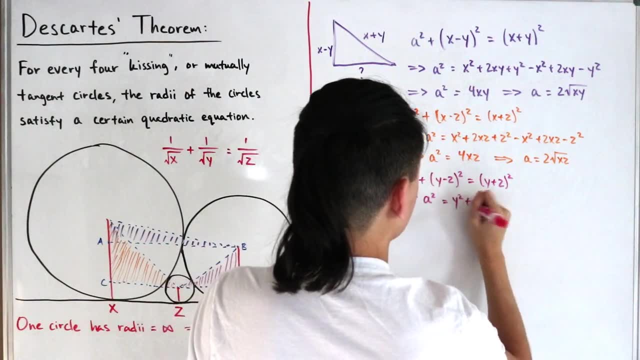 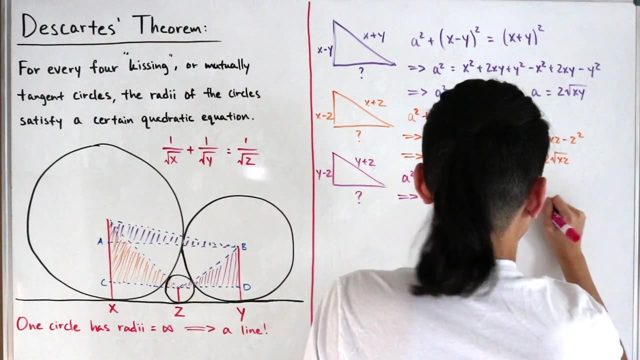 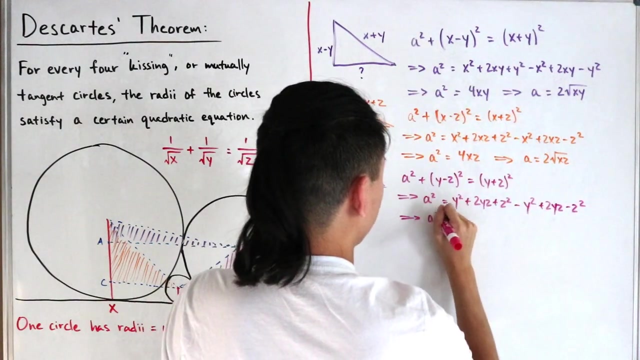 to uh y plus z square. Okay, Expand this out Then: um a square, then it's equal to y square plus two y z plus z square. uh, subtract y square, Then a square is equal to four y z. Then solve for a: a is equal to two times the square. 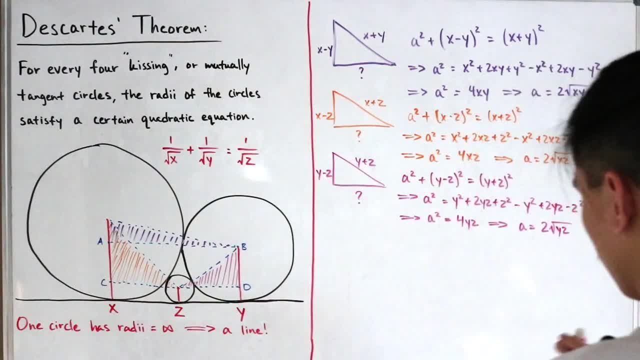 root of y times z. All right, So we have our bases. Let me just underline these, I'll box them. How about that? So we have the base for the purple triangle, We have our base- one of the bases- for the orange, and then we found our base for the pink, And then we 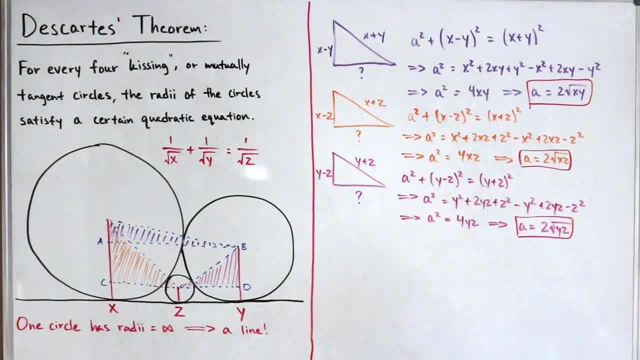 have our base for the orange, And then we found our base for the pink, And then we found our base for the orange, And then we found our base for the pink, And then we found our base for the orange. So let's actually do a little observation. Notice that um line. 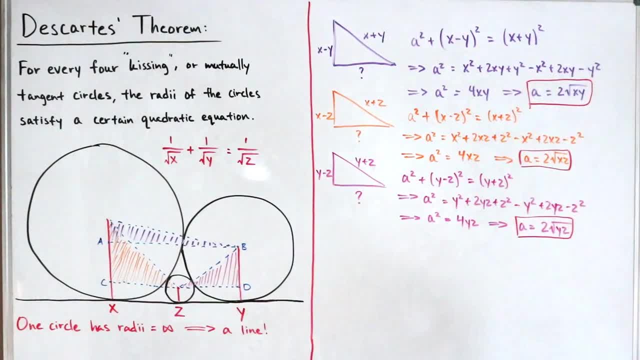 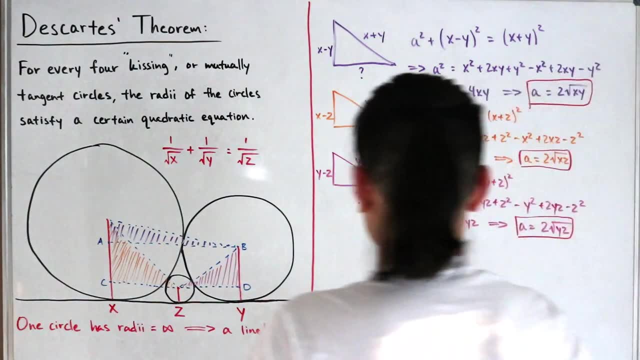 segments A to B and C to D. um, they're equal, since we actually constructed what is a rectangle, So those line segments are equal to each other, All right, So let's actually just wrote that. write that um observation. So noteall. 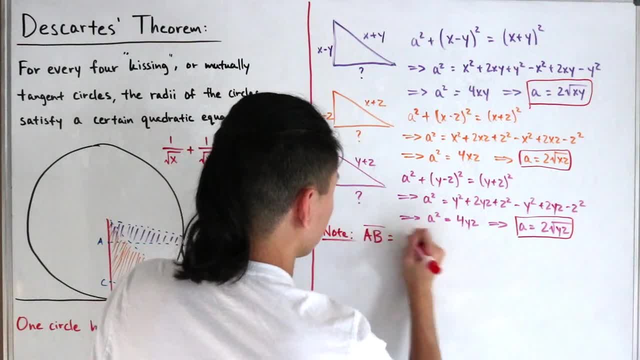 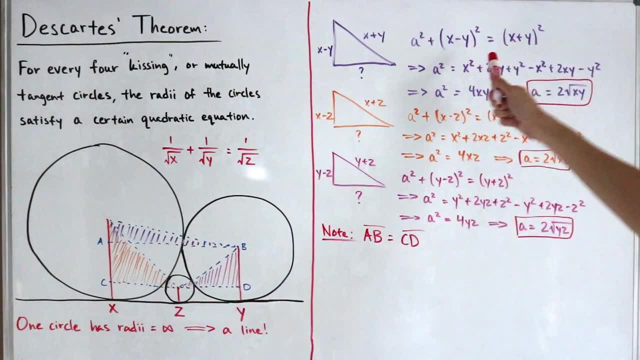 right Line segments AB is equal to the line segments CD. So what does lineso, what does line um AB equal to? Well, we just solved the base for the purple triangle over here in and we say that that base is just equal to two times. 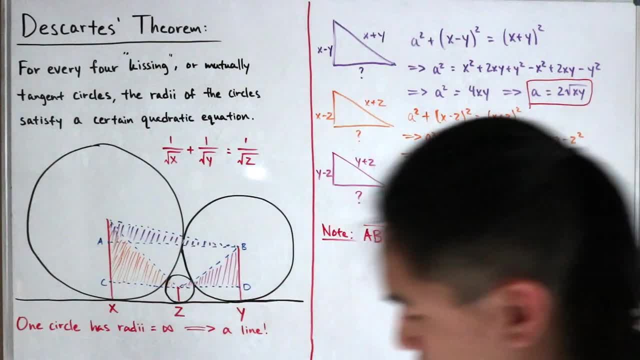 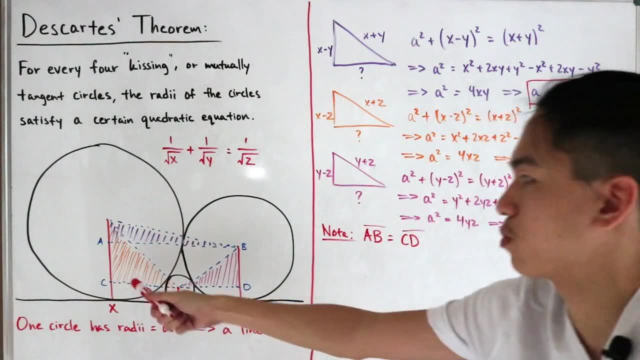 the square root of X times Y. So, and now the other part is, if we said CD is the line segment, so it's actually summations of our basis. See the purple triangle over here. it's base connected from Z to the center of our circle. 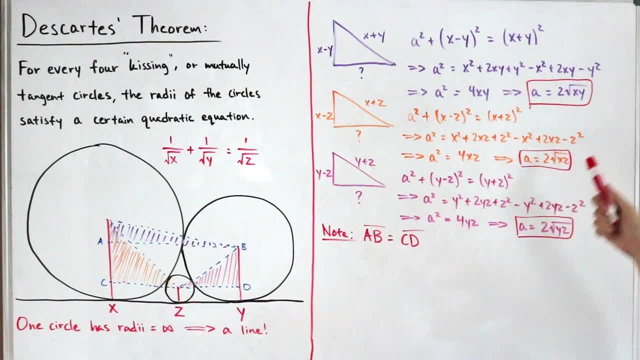 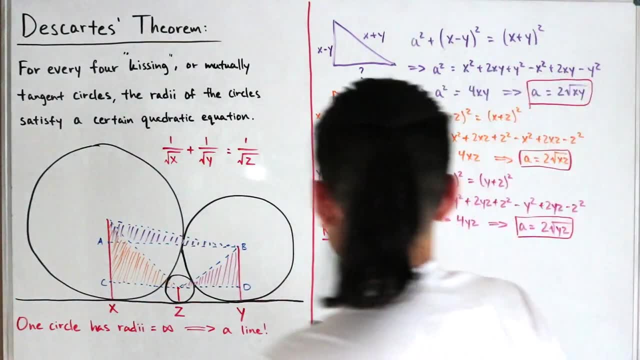 with radius Z, We said that that was equal to two times square root of XY. And then we add this with the base that we just saw for the pink triangle, which is plus two times the square root of Y times Z. So if I set these equalities to each other, 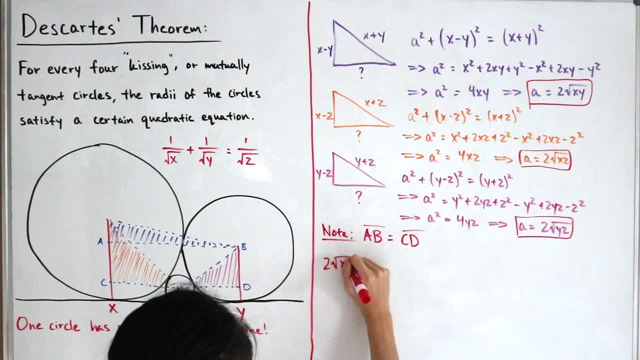 then we see that two times the square root of XY is then equal to two times X, two times the square root of X times Z, and add this with two times the square root of Y times Z. Okay, so now algebra time. we'll just divide two to both sides. 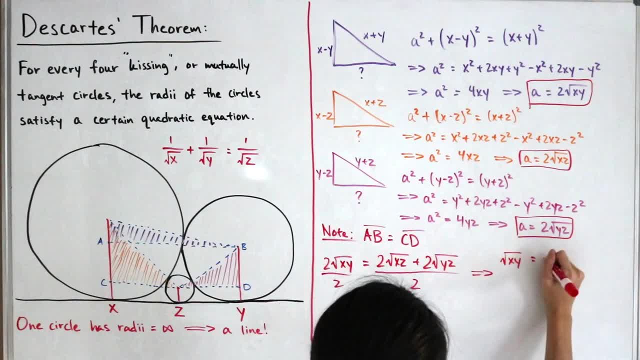 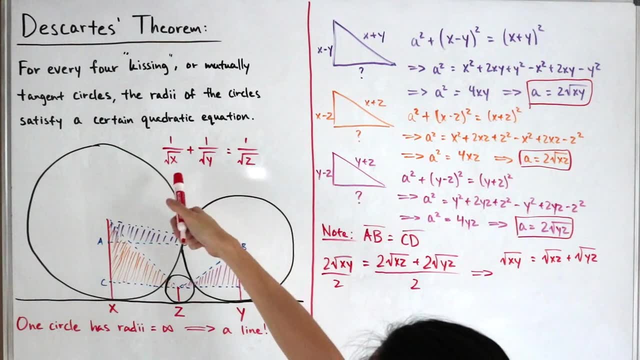 Then this is just the square root of XY equals square root of XZ. then plus two, plus square root of YZ. What we want to do is we want to prove that the reciprocal of the square root of the variables is equal to one over the square root of Z. 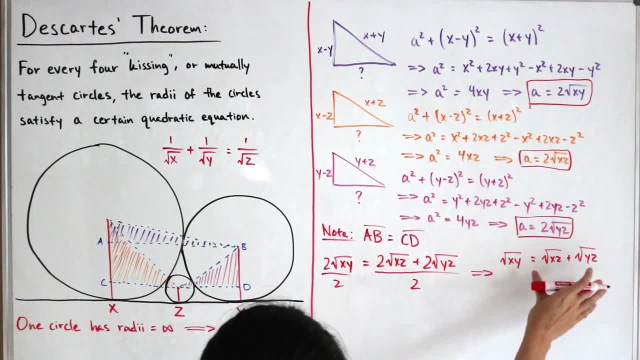 So let's actually do that and divide the square root of Z with both sides using the property of our square roots, that with the product it's actually just the square root of X times the square root of Z, for example, in this case, 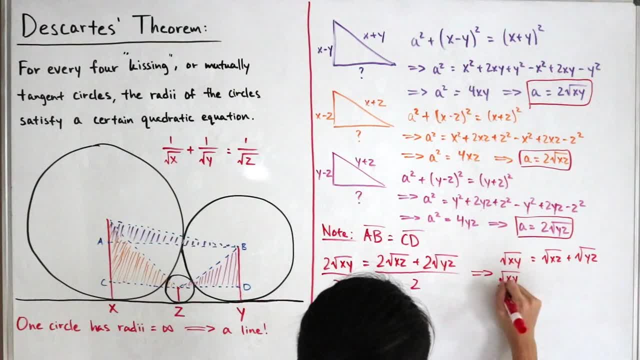 So when we do this square root of XY, square root of XY divided by square root of Z, Then that's just equal to How about this? And that's the case, if I'm defining the square root of Z, how about I divide the square root of XY? 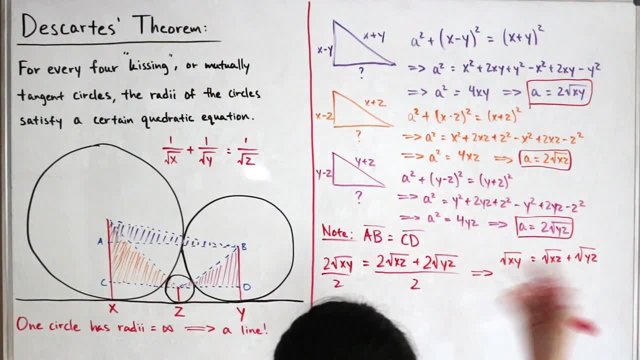 and then separate it out so the products, such that it's the square root of Xd times the square root of Y. So in other words, just doing this algebra, so it will just be one divided by the square root of Z, then that's just equal to. 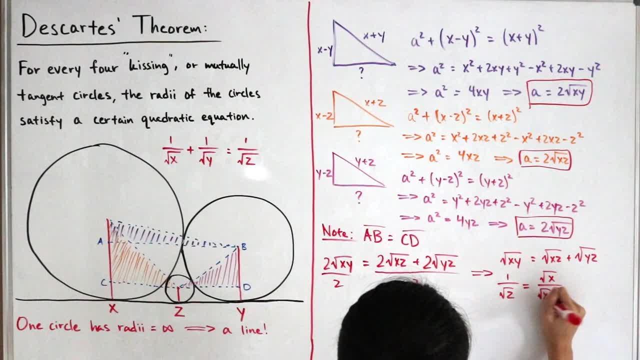 So it'll just be the square root of X than I divide it by the square root of X times the square root of Y, then add this with the square root of Y, y then divided by the square root of x times the square root of y. if we simplify things out. 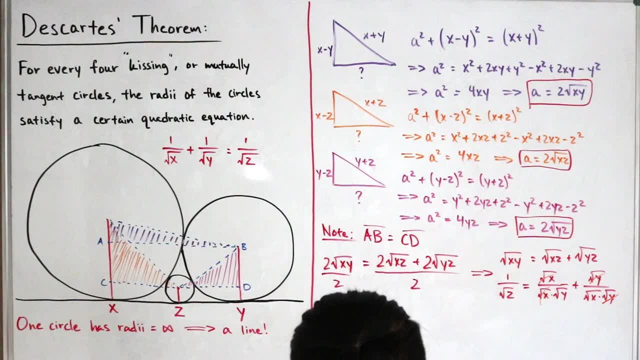 you'll see that that cancels, that cancels, and then that cancels, that cancels, and then we're actually just about done so. therefore, we've shown that one divided by the square root of z. it's just equality, it's just whatever. um, let's match. whatever you want to go with is actually just. 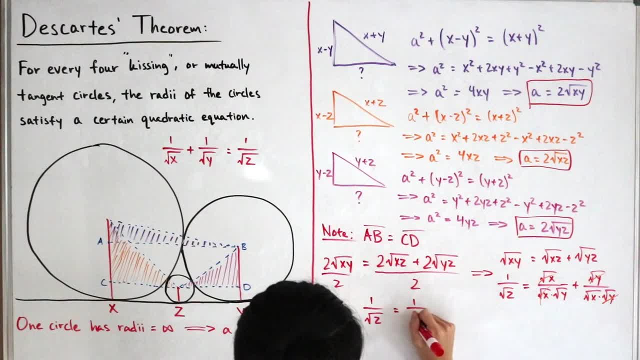 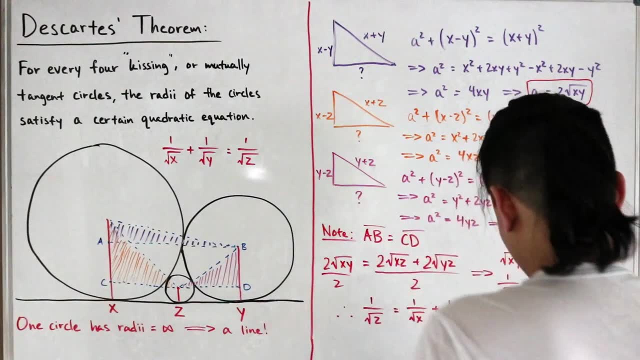 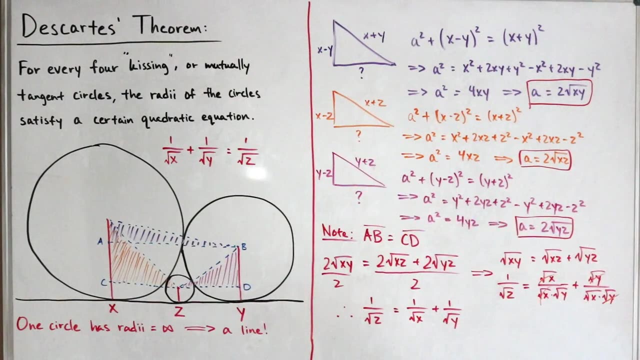 equal to one and it's addition, so it's commutative. so i can just write uh, square root, square root x first, and then add this with one divided by the square root of y, like so, and there we have. we proved the little geometry problem. uh well, the geometry theorem in a special case, such that our